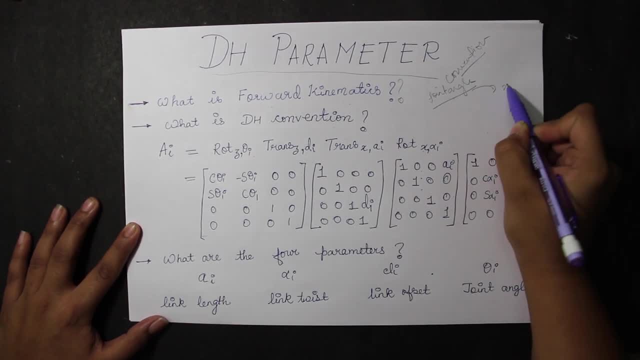 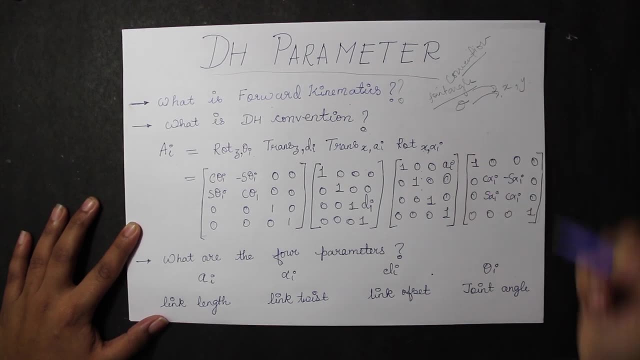 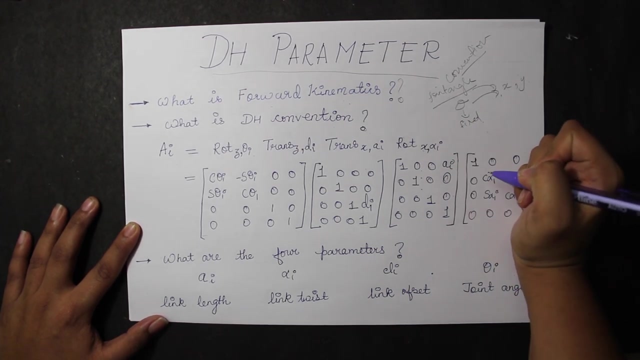 the individual joints of the robot manipulator and the position. Forward kinematics links the theta of the manipulator with the position it needs to reach. In forward kinematics, we give out the theta values of the manipulator in order to reach the position. That is the 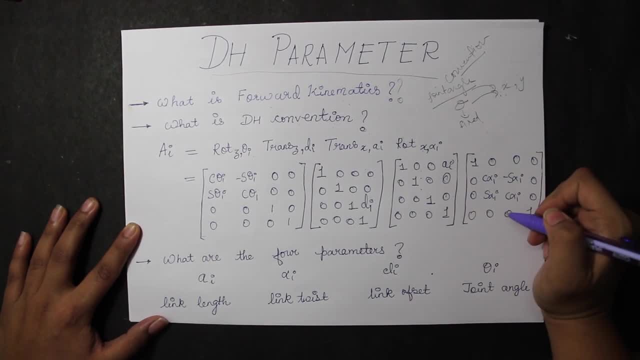 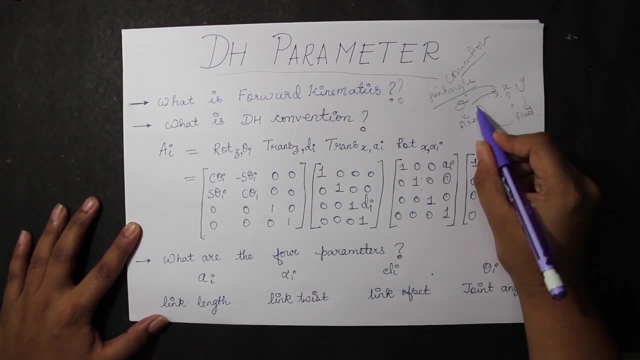 theta value is fixed and the position is what we are going to check, Whereas in inverse kinematics we define the position where we want to reach and instead we calculate the theta values of the manipulator. Now let us look at what DH convention is. 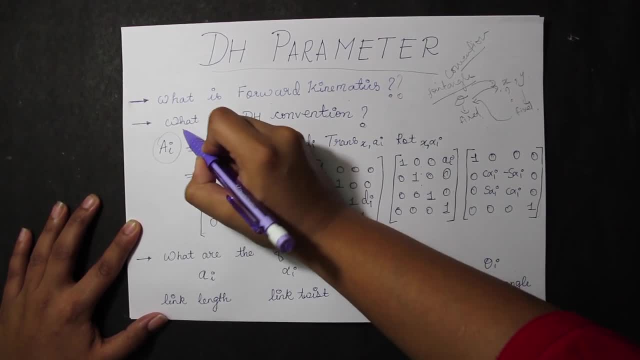 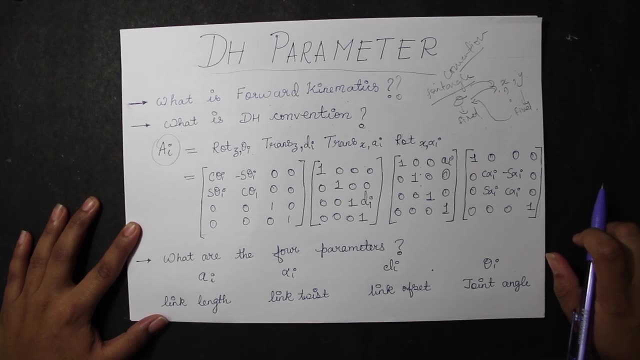 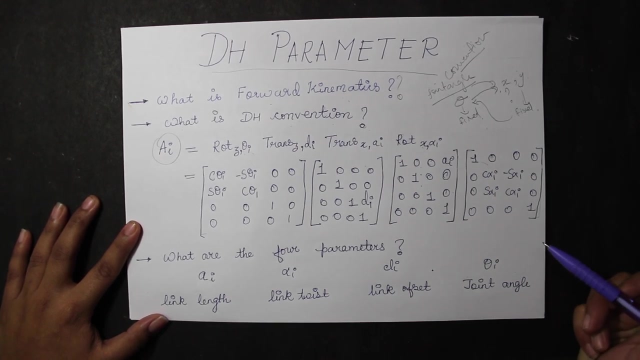 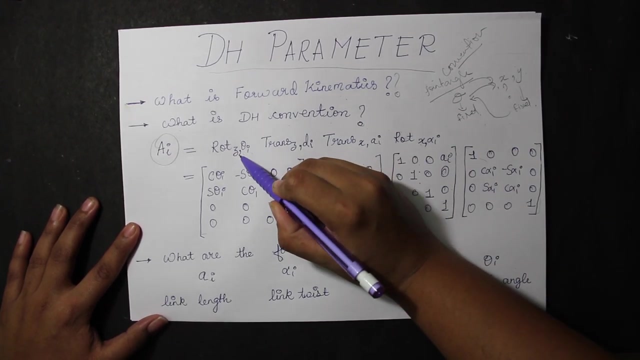 This convention links the homogenous transformation AI with the four basic transformations to find out the forward kinematics. So if we know the four basic transformation of the manipulator, we can find out its forward kinematics. What are the four basic transformations? That is, rotation at an angle of theta with respect to z, then translation along z for a value of di. 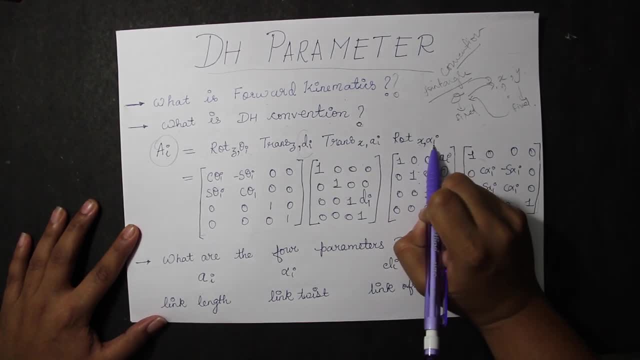 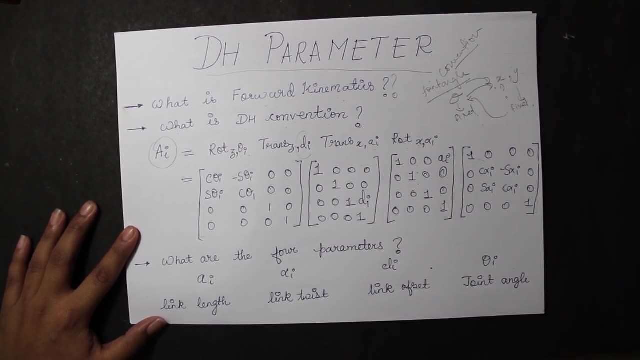 And similarly, rotation of x for an angle of alpha and translation of x for a value of ai. So now, what are those four parameters? That is, what is ai, what is alpha i, what is di and what is theta i. 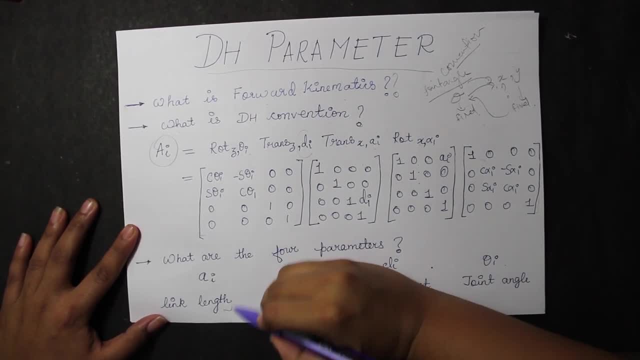 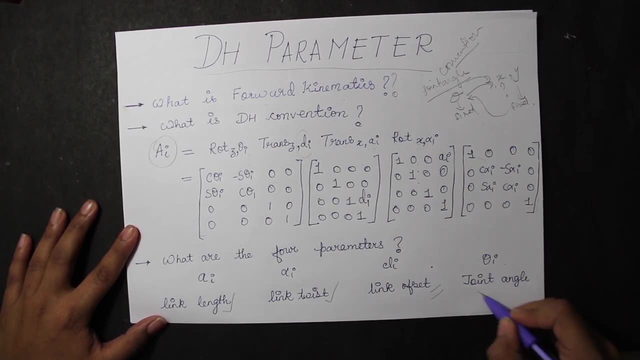 ai is the link length of the manipulator, Alpha i is the link twist, that is the angle it will move. di is the link offset and theta i is the joint angle between the two, that is, when a manipulator has two links, the angle between them. 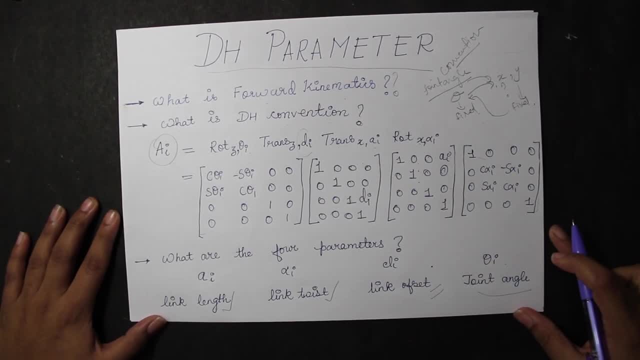 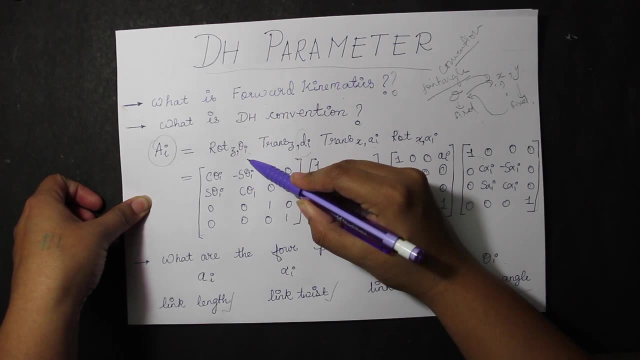 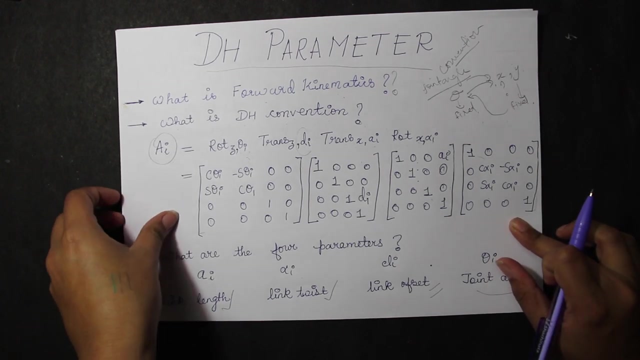 So now let's finally derive the rotational matrix. We have here rotation of z for an angle of theta i. I have already taught you how to attain this and all the four metrics. similarly, When we multiply all the four matrices, we attain to a formula comprising of ai, alpha i, di and theta i. 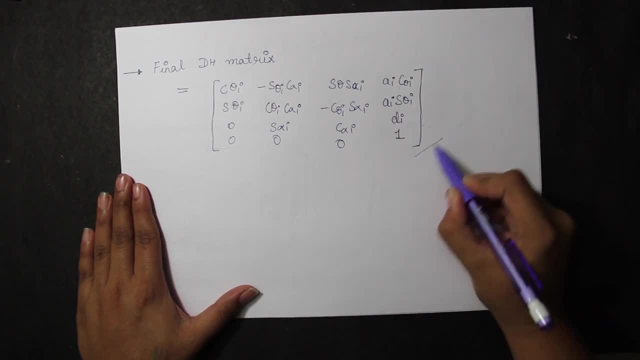 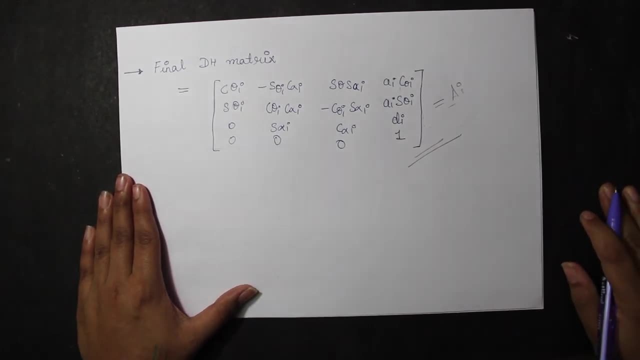 This final matrices is known as the homogeneous transformation, ai, and it's also known as the d-h matrix. When you multiply it, you'll get something like this: I would recommend that you go ahead and solve it on your own to get a better insight into it. 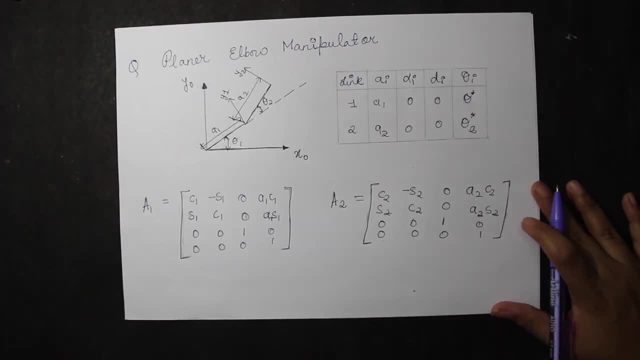 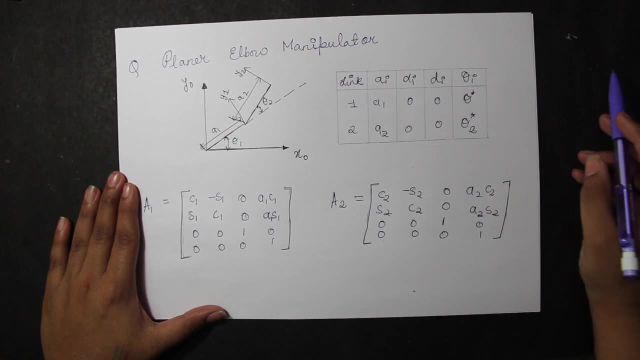 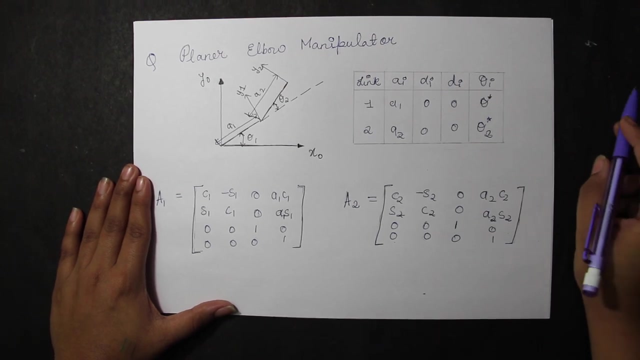 Now let's look at the parallel elbow manipulator. We have already derived the forward kinematics of this with the geometrical approach. Now let's look at a more basic and more fundamental approach of the d-h convention. So let's start. 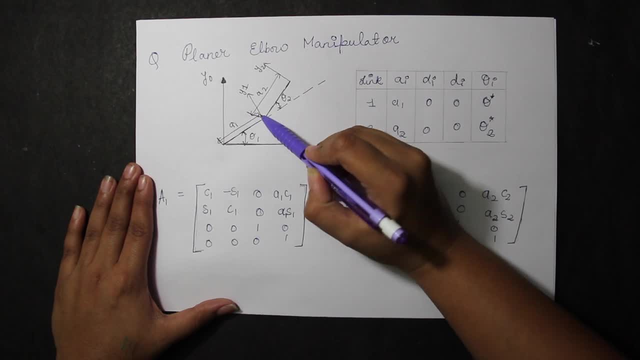 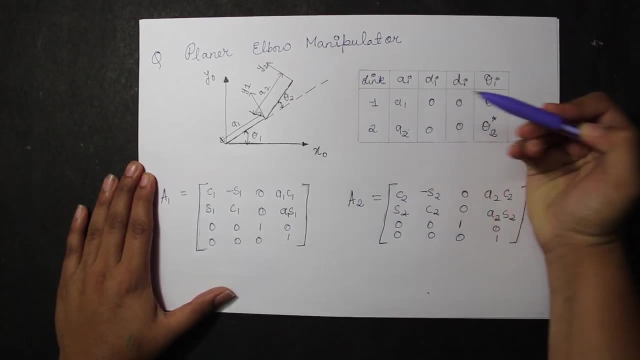 We here know that the link length for the manipulator is a1 and a2. That is, for link 1, it is a1 and for link 2, it is a2.. When we go to find out the link twist, 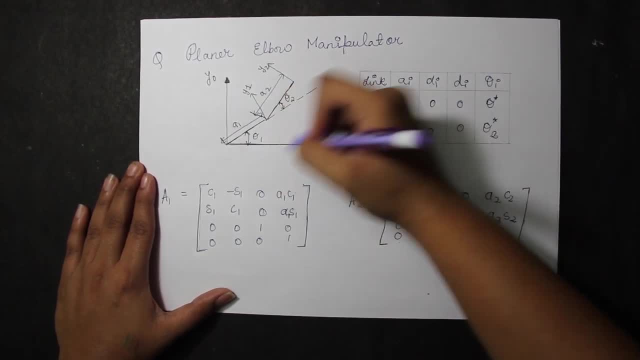 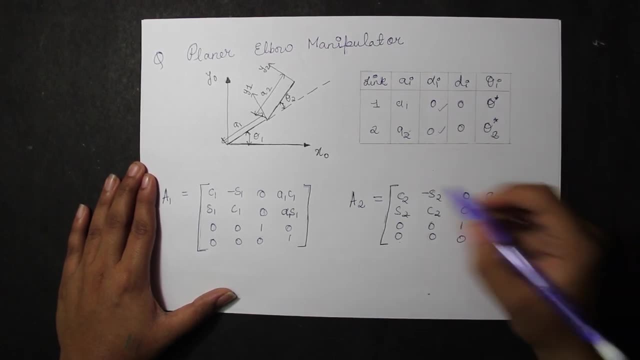 here. basically, we don't have any link twist, since it's basically defined at that position, So we define it as 0 and 0.. Similarly, we don't even have a translation of both the links and we have d1 and d2 as 0. 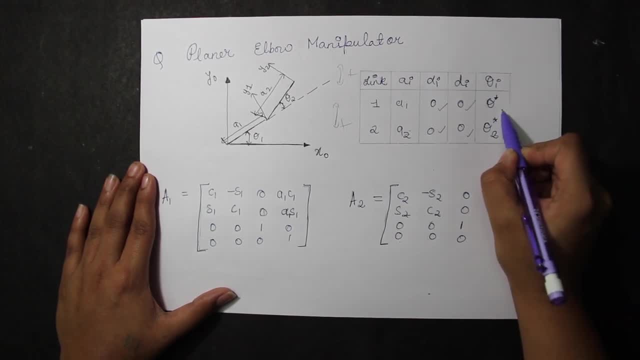 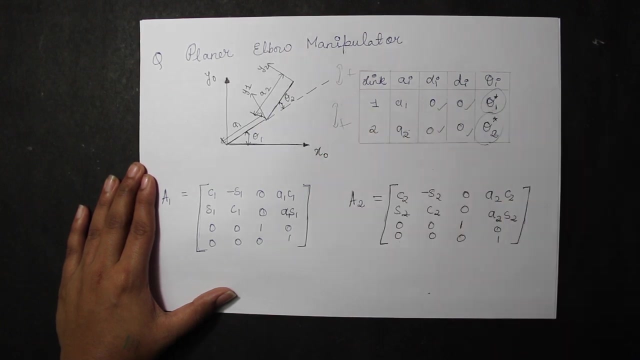 What we have here is the joint angle, that is, joint angle between the links, That is, theta1 between a1 and x-axis and theta2 between the originals a1 and a2 link. When we put it into the both-link formula, that is: 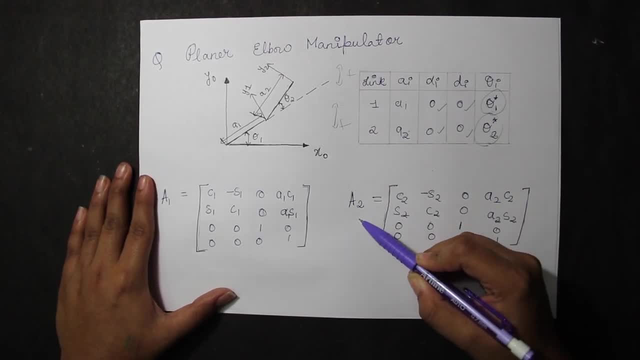 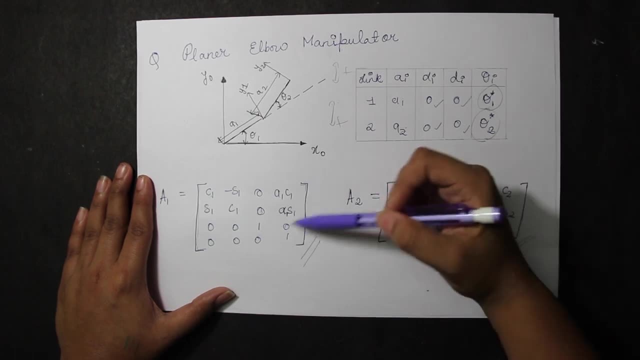 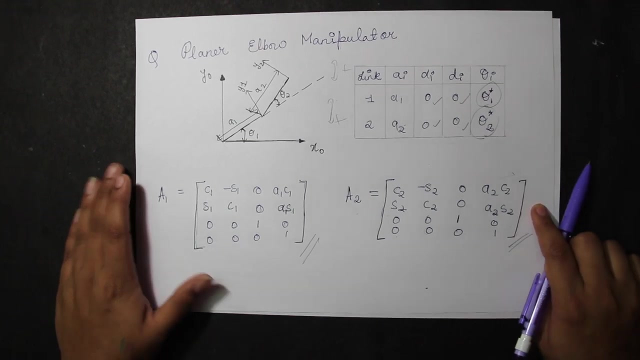 a1- homogeneous transformation- and a2- homogeneous transformation. you simply put the values of, that is, cos theta 1 sine theta 1, a1, cos theta 1, alpha 1 sine theta 1, and similarly for cos theta 2 sine theta 2, and so on. when you receive this, both the matrices a1 and a2, what we need to do 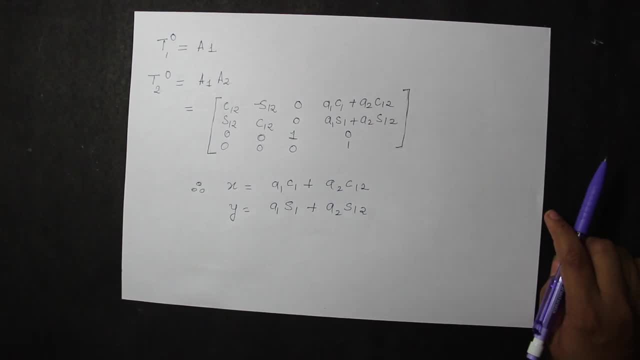 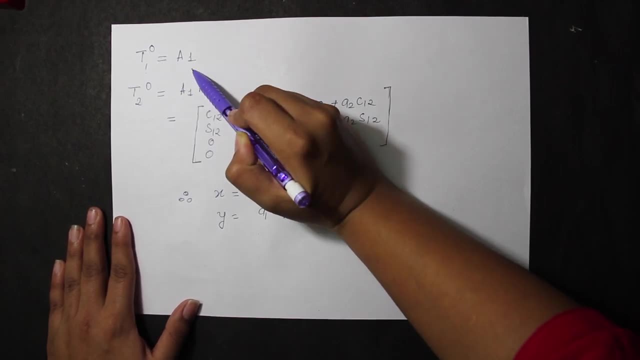 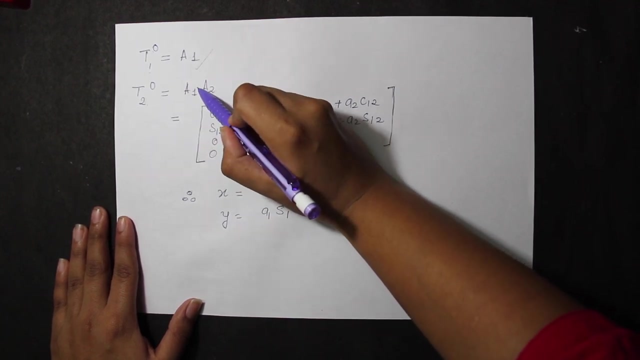 to find out the forward kinematics is really important. we know that t1 with respect to the zeroth frame is a1 because it's a homogeneous matrix, but we want to find out when t2 with respect to the zeroth frame, it'll be t1 with respect to zeroth frame and a2. that is our. 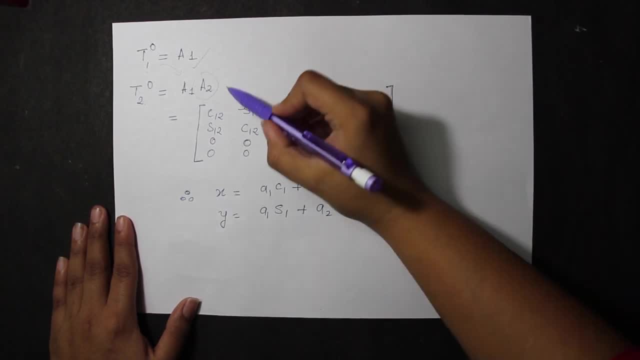 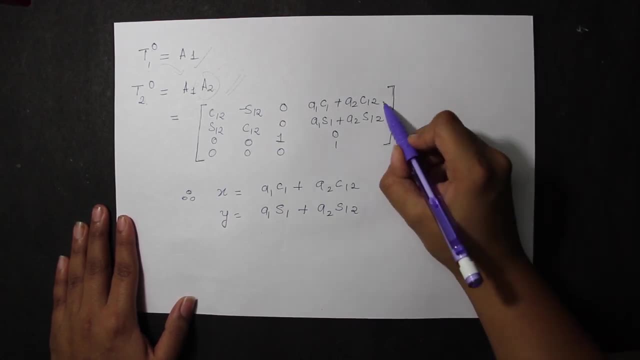 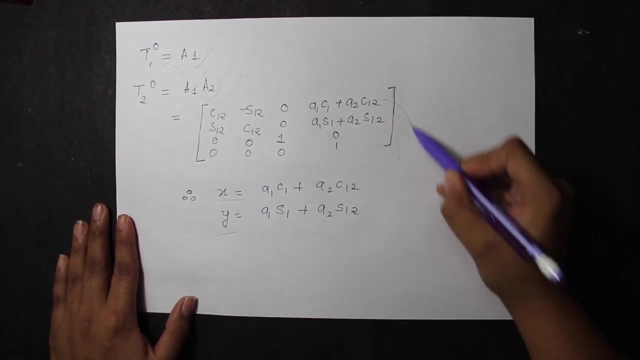 final matrices will be a1 into a2. you go ahead, solve it on your own and find out this matrices. when you find out this matrices, you will understand that forward kinematics for x will be a1 cos theta 1 plus a2 cos theta 1 plus theta 2, and for y it'll be a1 sine theta 1 plus a2 sine.